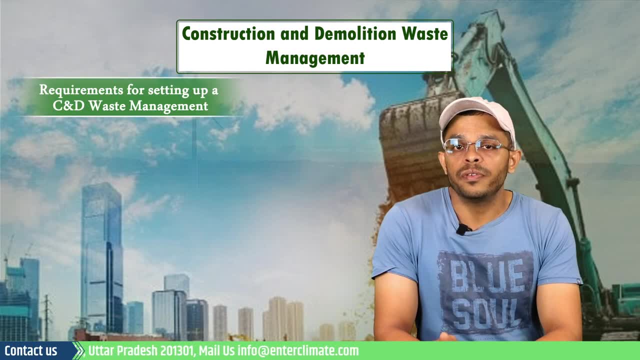 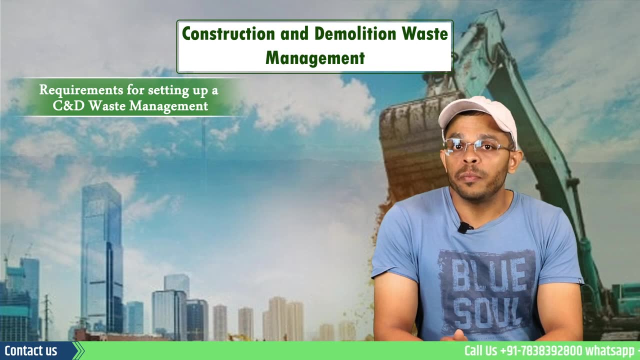 Let's see the requirements for setting up such a construction and demolition waste management facility. So many of these construction and demolition waste management facilities are being established in a PPP mode And they need a robust network of stakeholders Like builders, contractors, waste collection centers, urban local bodies, etc. 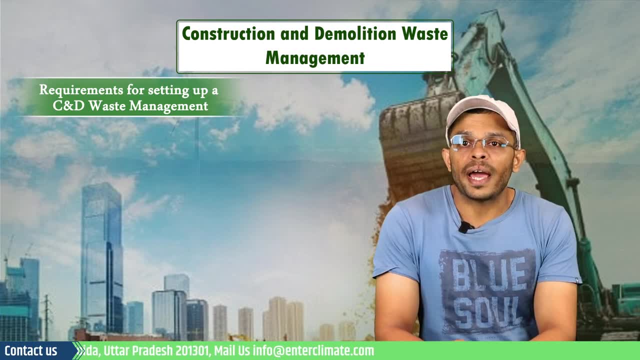 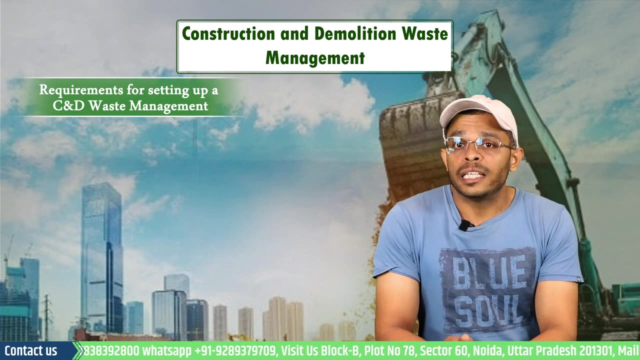 So, apart from the tie-ups with urban local bodies for managing waste in a city, the operator of such facilities must also coordinate with other waste management facilities, like bulk waste recyclers and waste processing facilities dealing with components recovered from C&D waste, As mandated by the 2016 rules. the project proponent must ensure that the processing 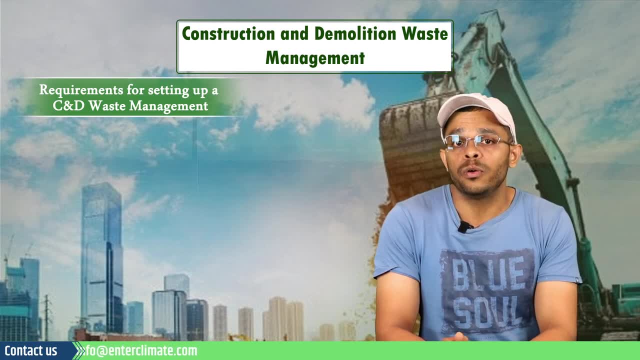 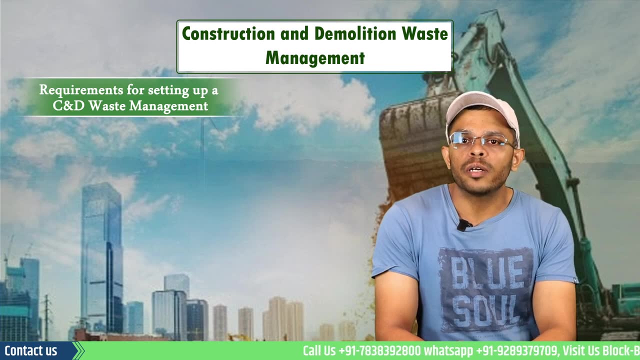 or recycling facilities are properly managed. The recycling facility must be large enough to last for around 20-25 years. The recycling site must also be away from habitation clusters, forest areas, water bodies, monuments, national parks, wetlands, etc. 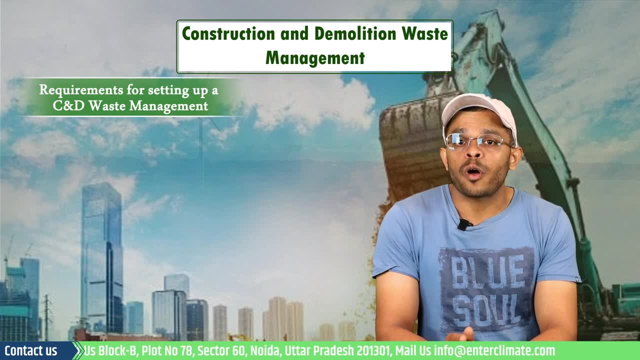 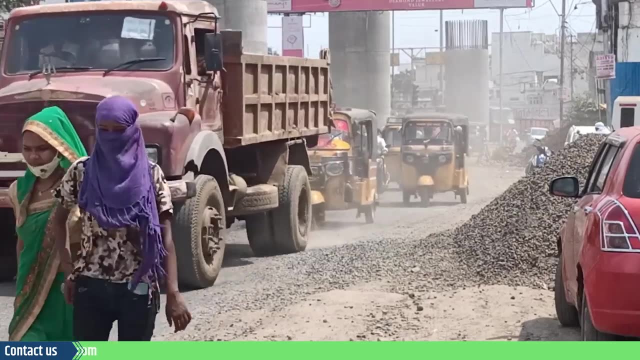 The site must be fenced or hedged and provide a proper gate to monitor incoming vehicles or other modes of transportation. The approach road and internal roads must be concreted or paved to avoid generating dust particles due to vehicular movement. The recycling site must be large enough to last for around 20-25 years. 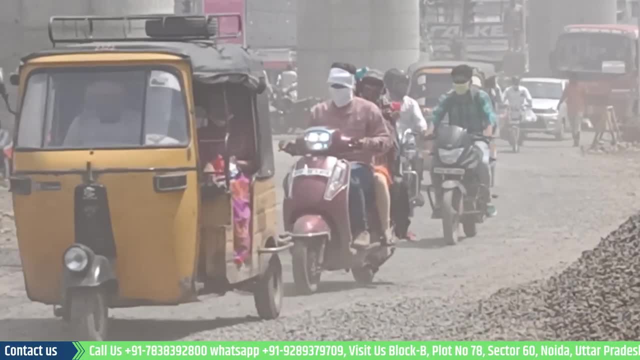 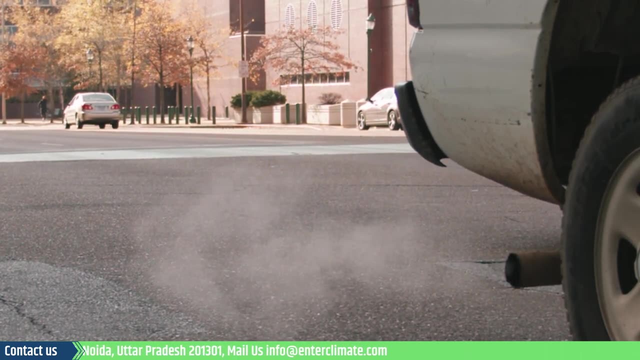 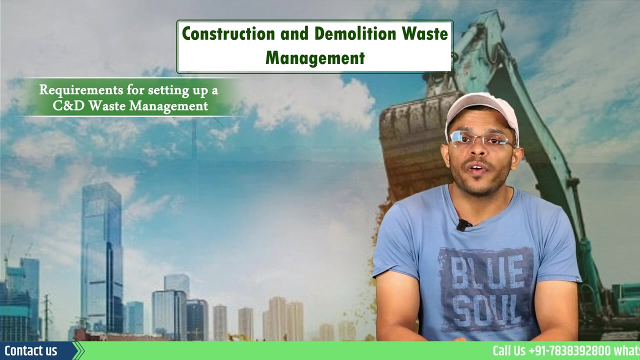 The site must be designed in such a way to ensure that unobstructed movement of vehicles and other machinery is possible. A weighbridge must also be installed to measure the quantity of waste brought to the landfill site. Fire production devices and other facilities as may be required must also be provided. 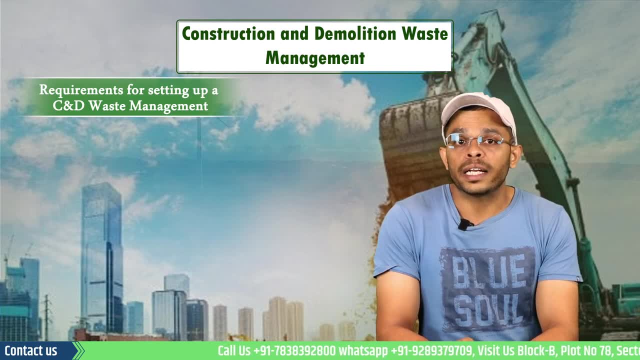 As well as provisions for stormwater drain to prevent stagnation of water surface must be installed. Provisions for treatment of effluents from the unit to meet the discharge norms as per the environment protection regulations must also be provided. The speed of production must also be decided based on the number of vehicles being imported. 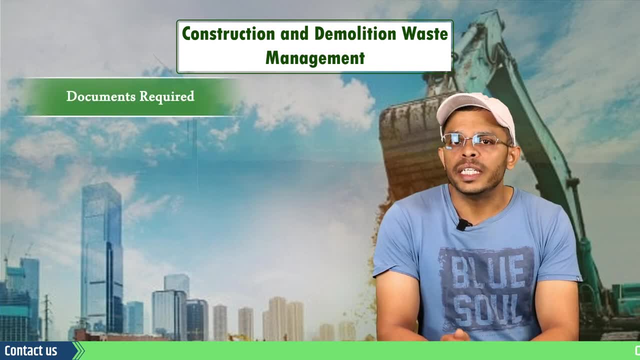 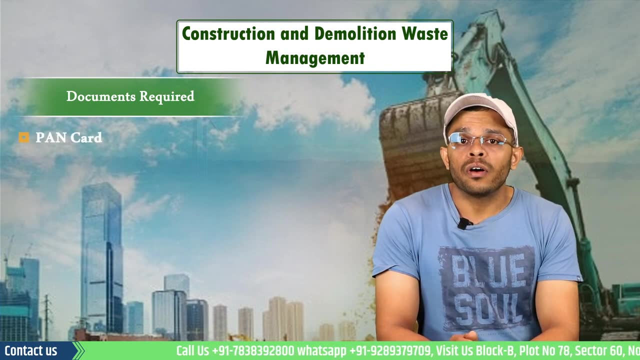 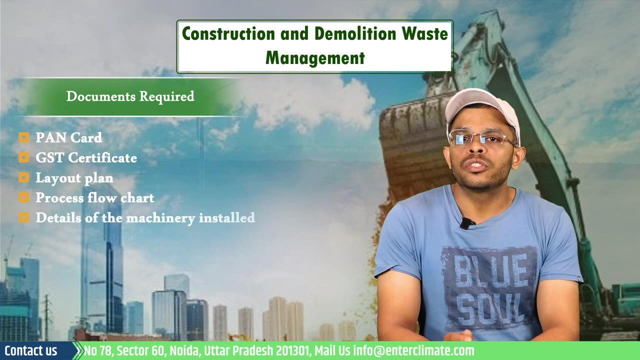 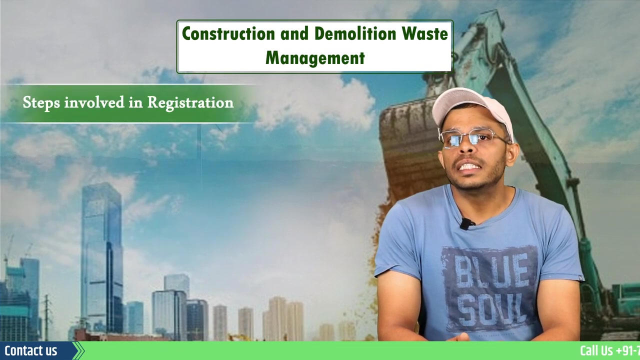 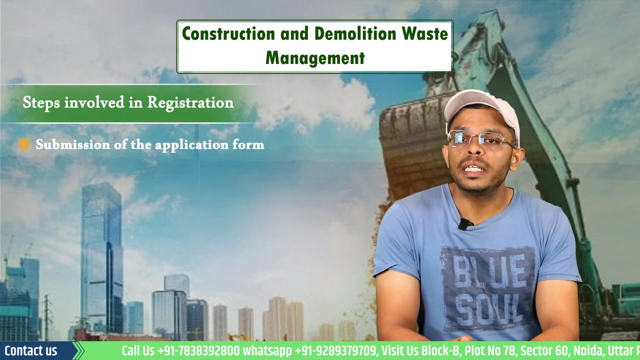 and as well as AttractionRPOT control. The site must be Spanish-tongued and the the first step is submission of the application form. here the documents and the application form is submitted to the concerned state pollution control board to set up a processing or recycling. 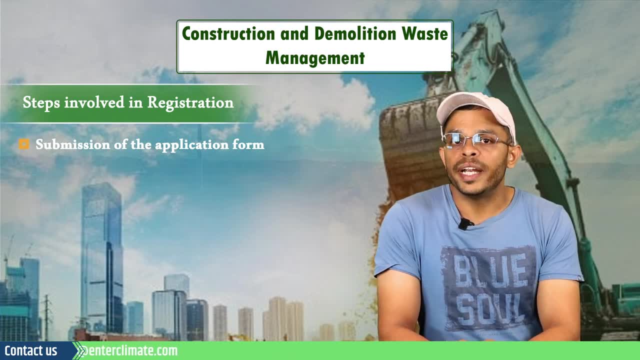 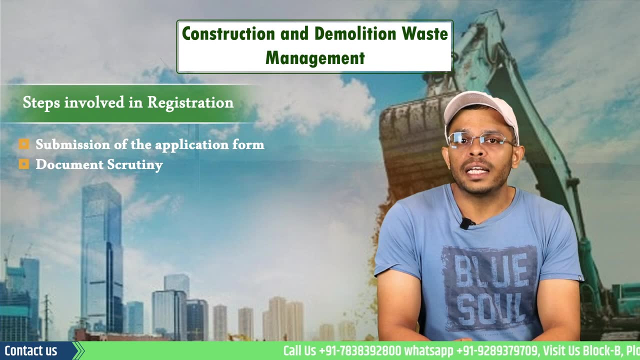 facility, an application in form 1 has to be made to the concerned spcv. the second stage is document scrutiny, where all relevant documents are scrutinized at the member secretaries level to assess the proposed sites capacity and disposal capacity. and finally, the last stage is the 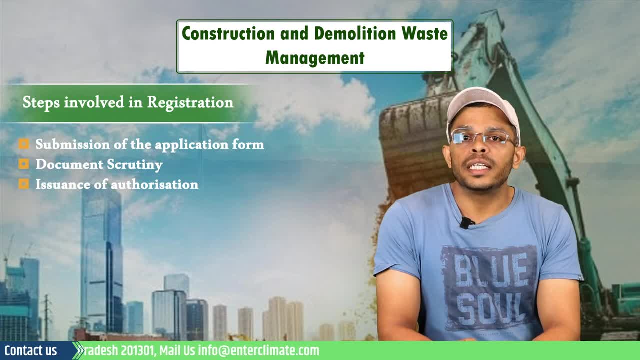 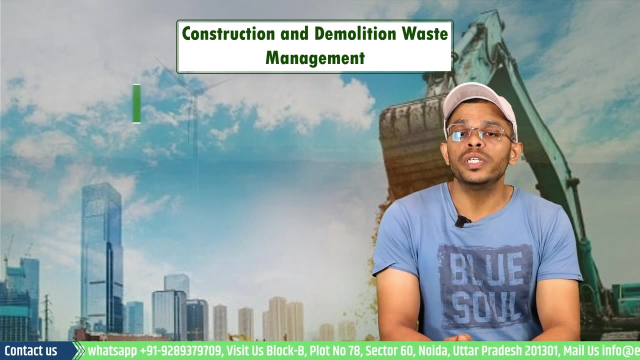 issuance of authorization. at this stage, the concerned state pollution control board will grant the license to the cnd waste management facility in form 3, as specified under the rules, after examining the application. so if you are looking to set up such a facility, you must understand the duties of the cnd waste management operator and the waste generator. let's first 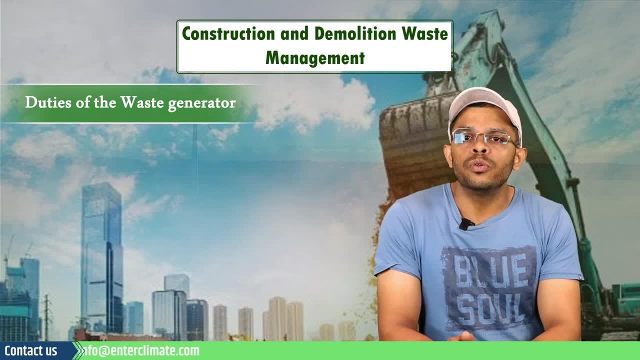 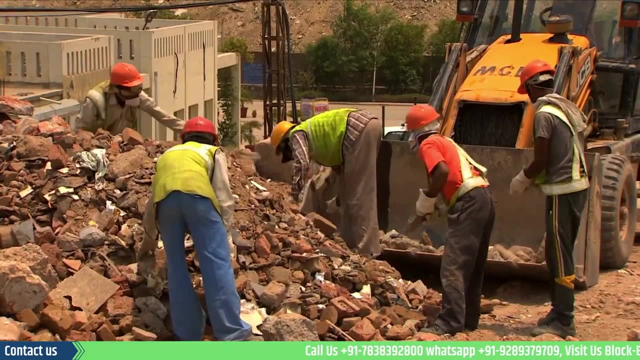 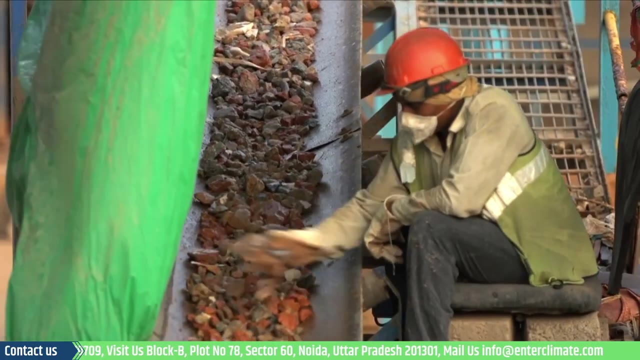 discuss the duties of the waste generator. the cnd waste includes surplus or damaged products and materials that arises during construction work and are temporarily stored on the site. many states are now recognizing the importance of processing cnd waste. a waste generator includes any person or their association institution. 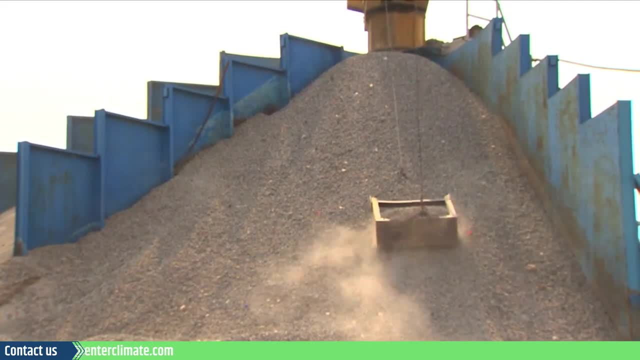 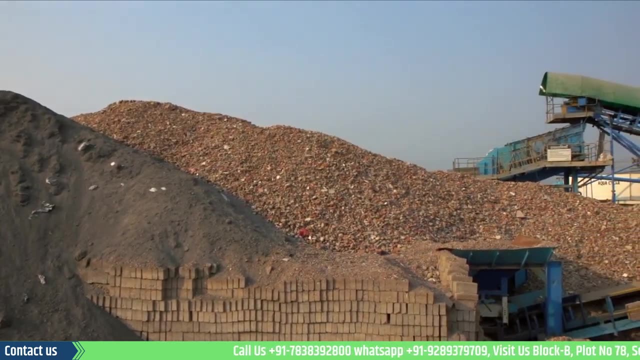 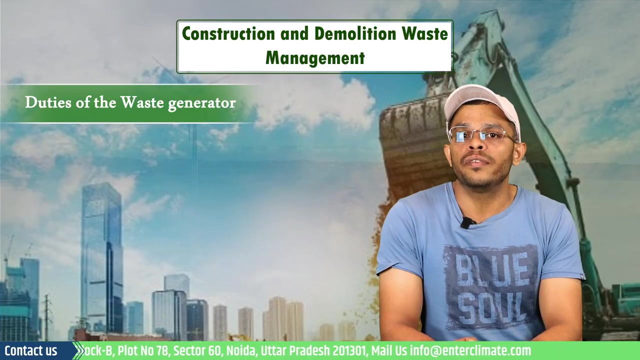 and commercial establishments like indian railways, ports and harbors, airports and defense establishments that undertake construction or demolition of any civil structure and generate construction and demolition waste. the generator of such waste should inform the concerned civic authority in writing before undertaking such activities and deposit the application fee. 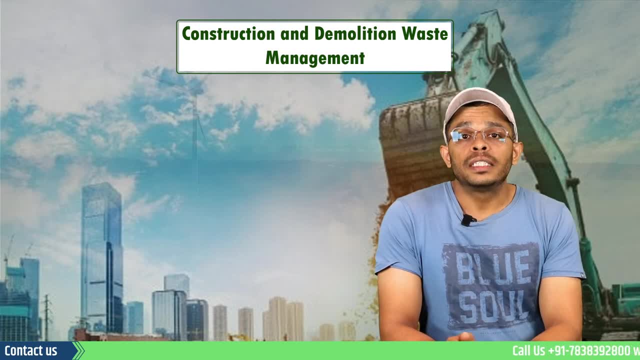 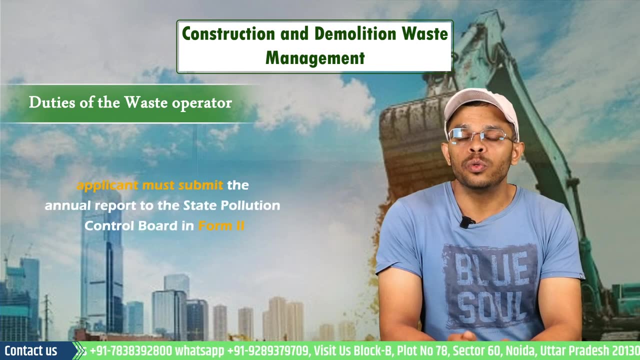 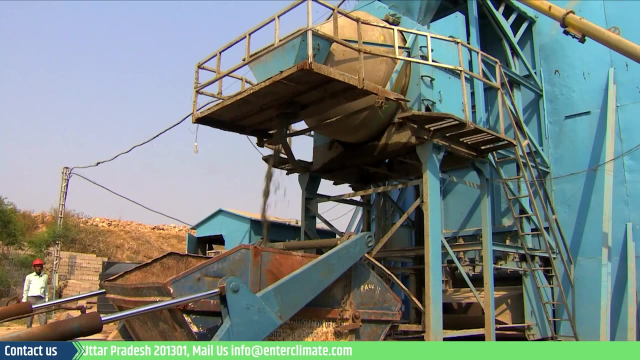 according to the notification of the municipality. now let's see the duties of the waste processor. so the applicant must submit the annual report to the concerned spcb in form 2 of the rules. the waste generator is responsible for the collection, segregation of concrete, soil and other. 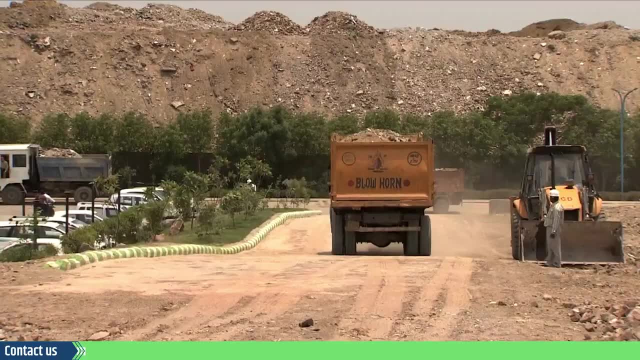 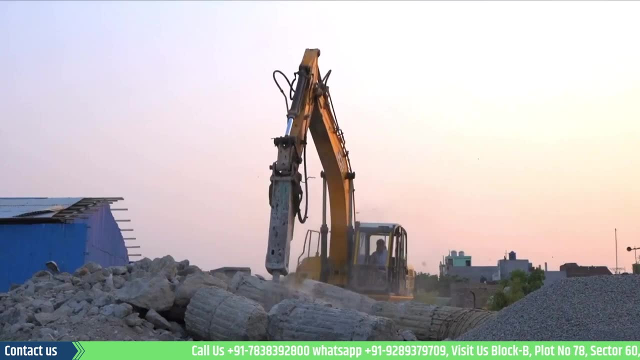 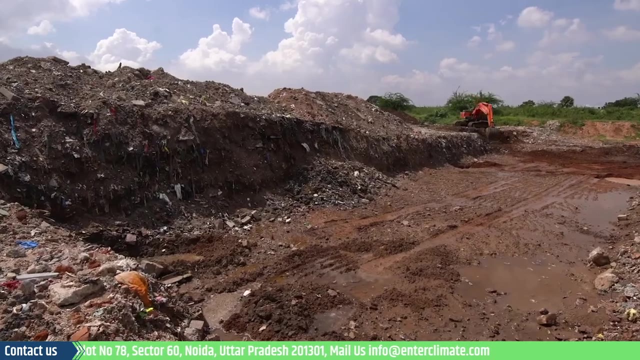 cnd waste generated as directed or notified by the concerned local authority. apart from this, the waste generator needs to fulfill responsibilities such as: ensuring that other waste is not mixed with the waste and is stored and disposed of separately. ensuring that if the waste generated is 20 tons or more in one day, or 300 tons per project in a month, he must segregate that waste. 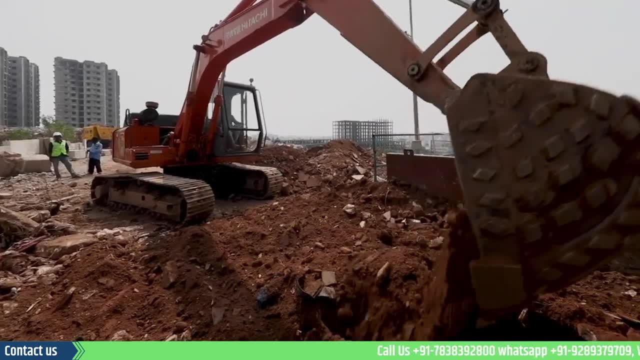 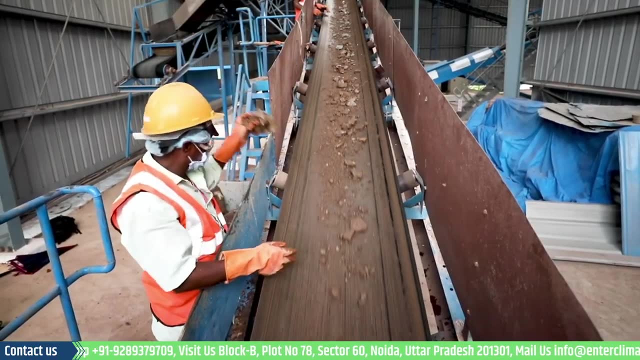 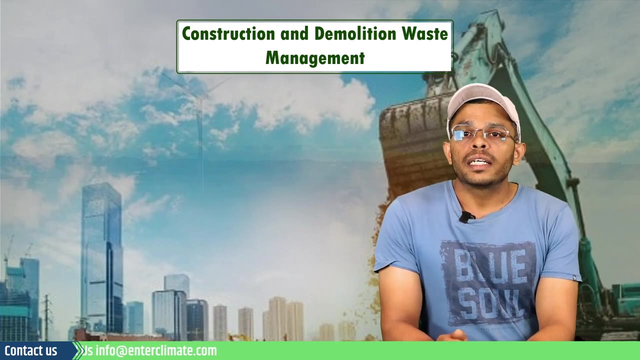 into four streams, that is, concrete, soil, steel, wood and plastic, bricks and mortar, and submit their waste management plans accordingly. he must also get appropriate approval from the local authority before starting such construction or demolition work, ensuring that construction and demolition waste is kept within the premises or gets deposited at collection centers under the.